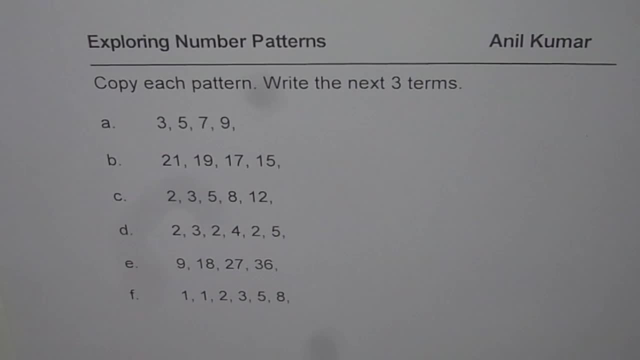 I'm Anil Kumar, and now let us explore some number patterns. We'll start with simpler ones and then have slightly more difficult as we move on. Copy each pattern. write the next three terms. You can pause the video. copy these patterns, right? So we have six of them for you. The first: 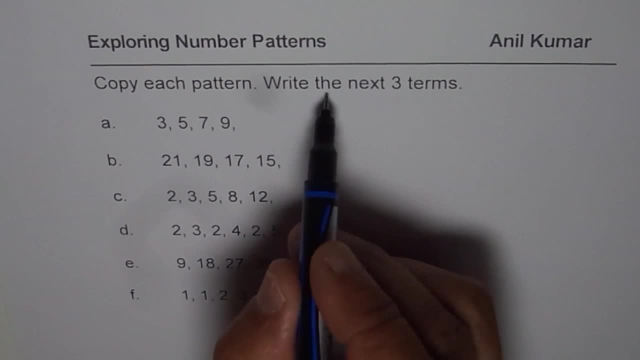 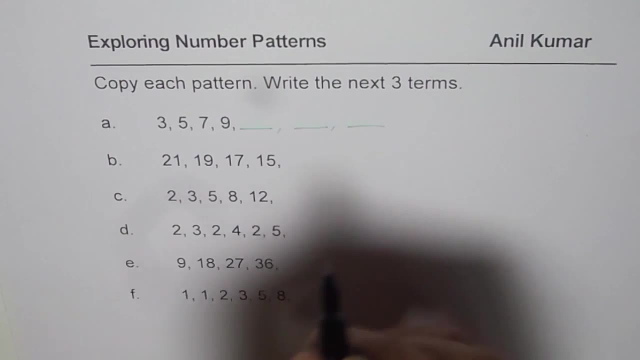 one is 3,, 5,, 7,, 9.. You need to write next three terms, That is to say what comes after 9 and then and these three terms correct. So likewise, copy each pattern and write next three terms. 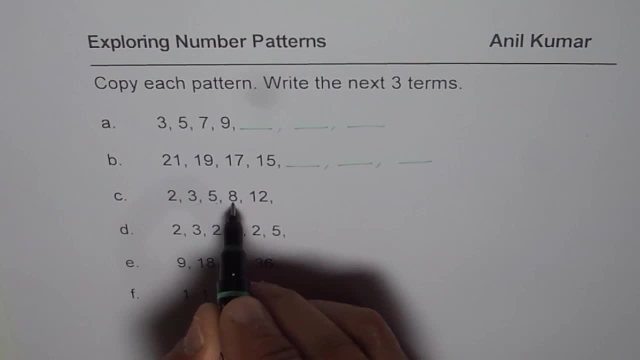 So we have now 2,, 3,, 5,, 8,, 12 and then next three terms: 2, 3,, 2, 4,, 2, 5,, next three terms, right? So likewise 9,, 18,, 27,, 36,, next three terms: 1, 1,, 2,, 3, 5, 8.. This is a bonus question, right? 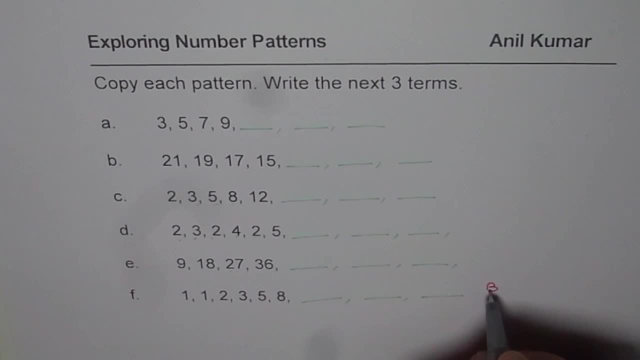 This is very difficult, So this is a bonus question for you. You can take anybody's help to solve this question, correct? So these are the number patterns which we need to explore now. Correct, Let's begin with the very first one. These are all. 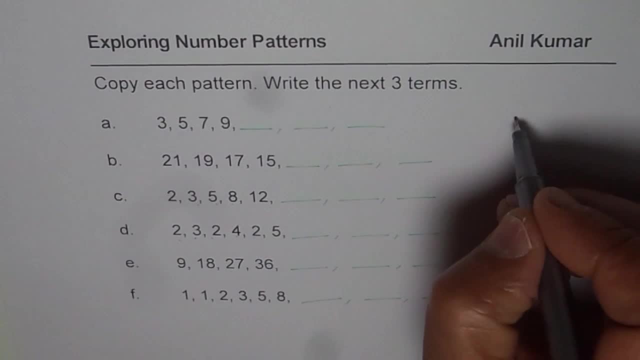 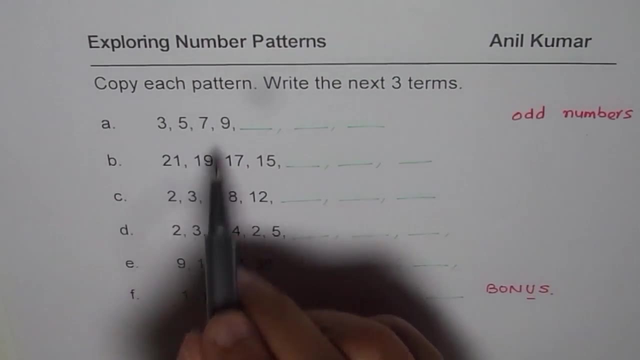 correct. Let's begin with the very first one. These are all correct. Let's begin with the very odd numbers. 3, 5, 7, 9 are odd numbers. right, These are odd numbers. And the skip counting. Do you see the skip counting? Add 2 each time. So next term, you. 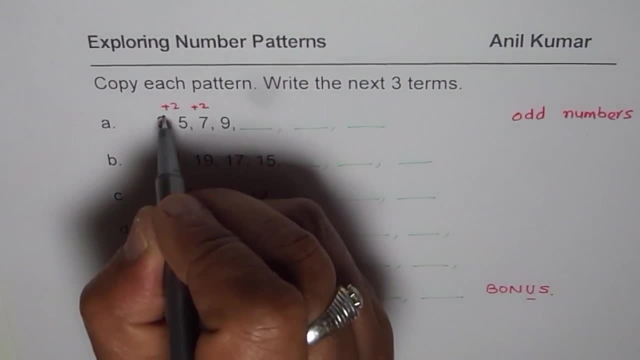 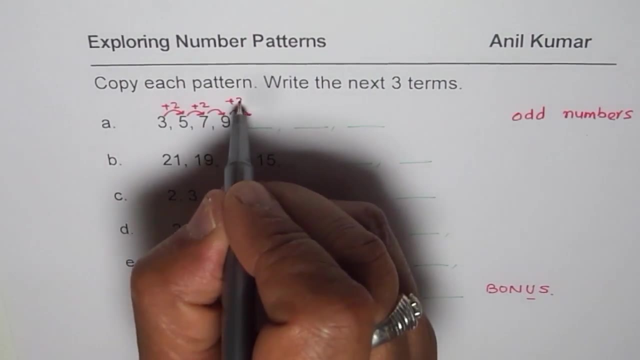 get by adding 2.. So add 2 each time correct To get to the next number. So that is how you can figure out. So next number should be 9 plus 2. That is to say 11. And then we have 13,. 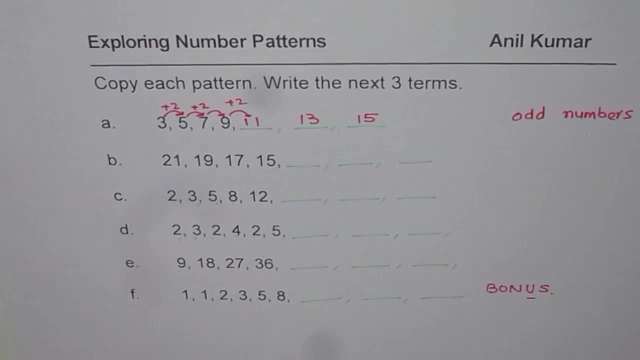 14, 15.. So that is how you get next three terms. Now let's look into part B: 21,, 19,, 17, 15.. Well, what we need to see is: it is decreasing, correct. It is a decreasing pattern And it is decreasing. 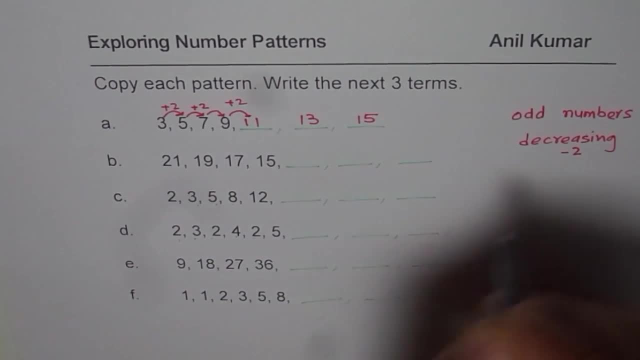 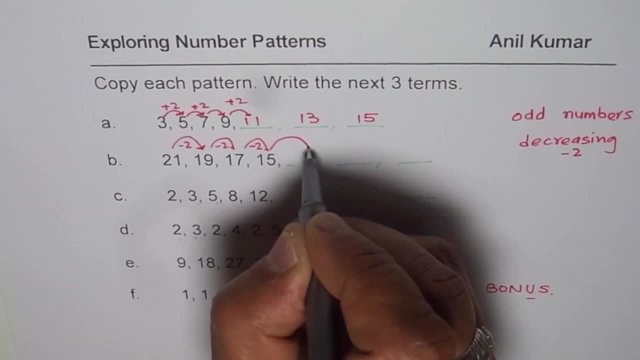 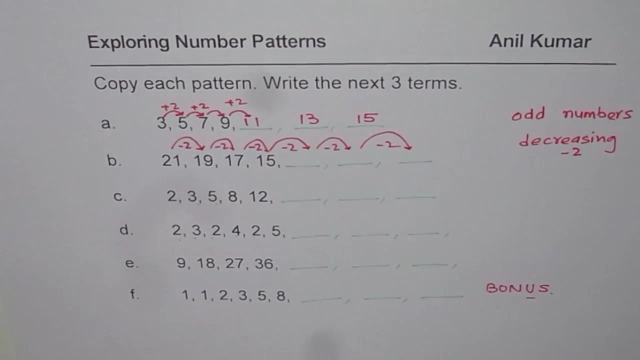 minus 2 to get to the next term. So to get here, we have to do minus 2.. Again, we have to do minus 2.. And then again take away 2 to get the next term. So let us take away 2 each time, So 15. 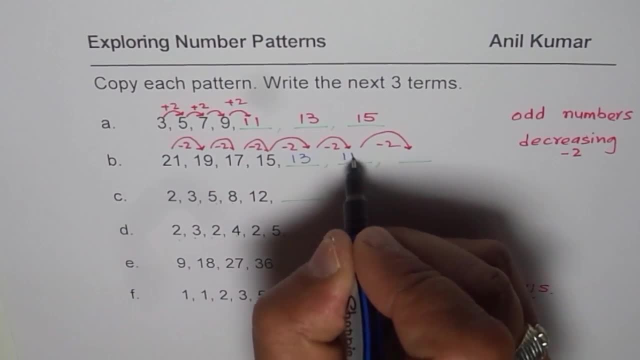 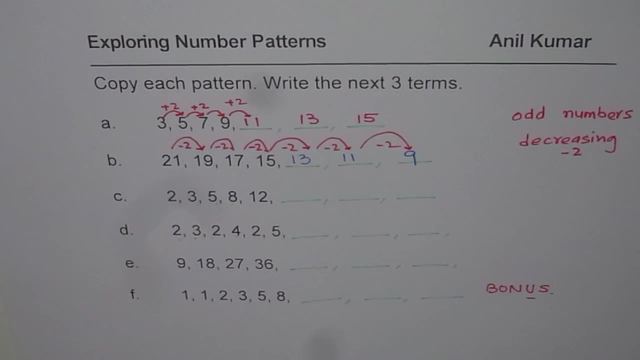 take away 2 is 13.. 13. take away 2 is 11.. 11. take away 2 is 9.. Next one is 2,, 3,, 5,, 8,, 12.. Now how to do this one. 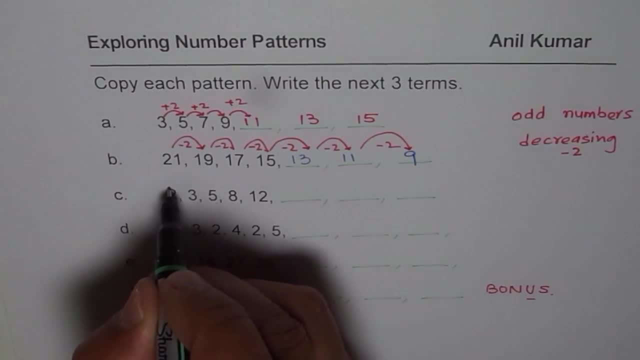 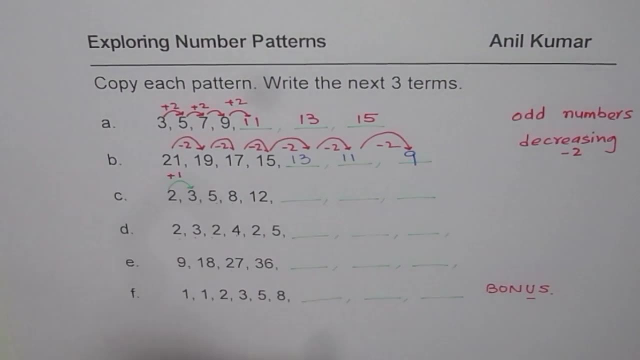 It is kind of tricky. So when you move from 2 to 3, you add how much, You add 1.. So it is plus 1, right, 2 plus 1 is 3.. But when you move from 3 to 5, you are adding 2, right, You are not adding 1,. 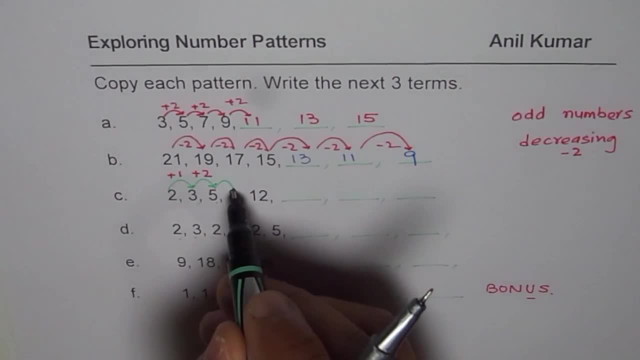 but you are adding 2.. So when you move from 5 to 8, you are adding 3,, right? So it is plus 3.. And then, if you do plus 4, do you get 2?? So you get 2.. So when you move from 5 to 8, you are adding. 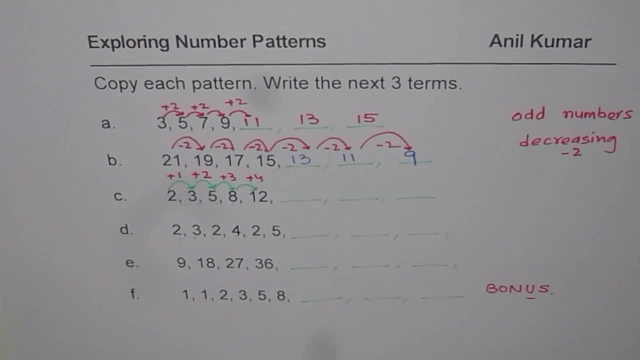 3. And then, if you do plus 4,, do you get 12? Yes, you do, Correct. So you add 1 more each time. So here you add 1 more each time. Do you see that? So that is the type of pattern you have. You start. 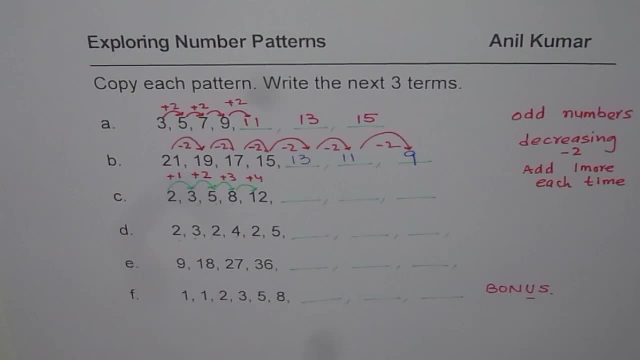 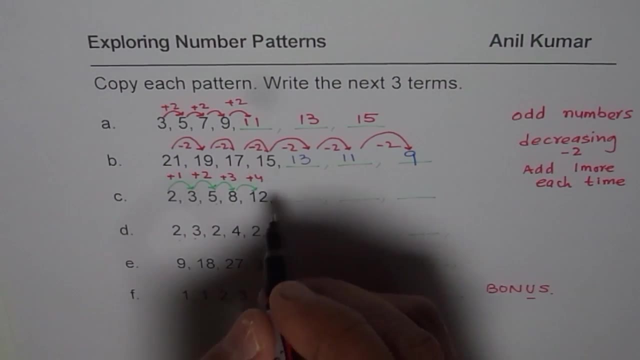 at 2,, add 1, and 1 more each time. That is what the pattern is. Now we know the pattern. Let us write down the terms. We will add 5 now. If you add 5, you will get 12.. So you add 1 more each time. 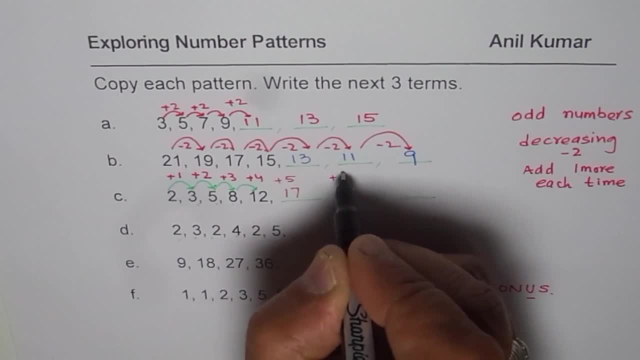 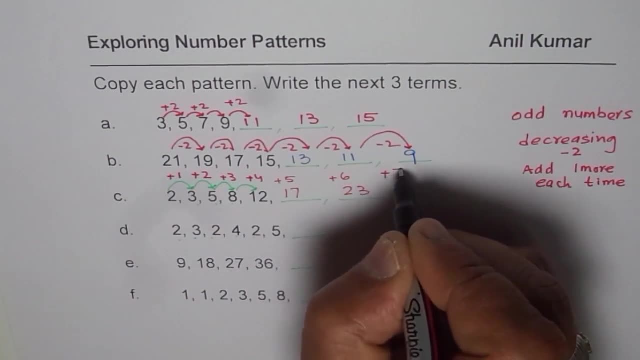 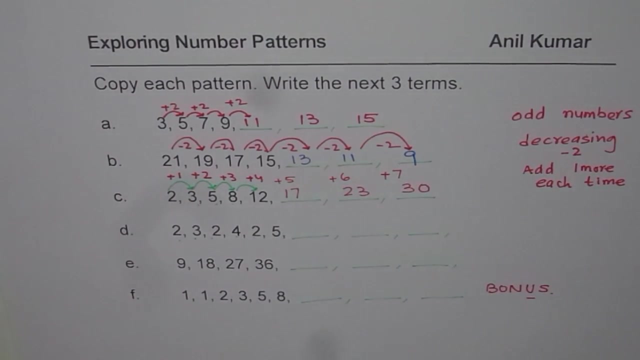 5,, you get 17.. Then we will add 6.. Do you see that? So 17 plus 6 is 23.. Now you add 7.. So when you add 7,, you get 30. Well, you can use the calculator or lines to add correct, So you could. 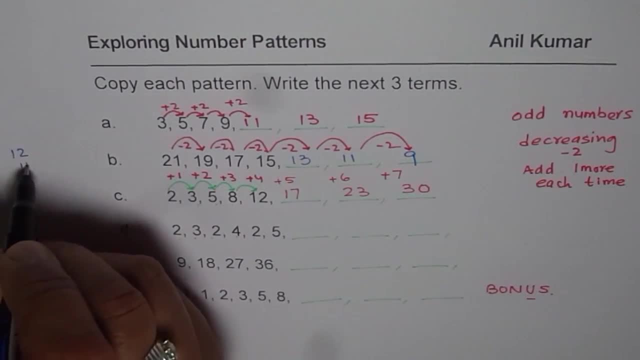 do 12 plus 5.. You could do 12,, and then 1,, 2,, 3,, 4,, 5.. 13,, 14,, 15,, 16,, 17.. So you get 17,. 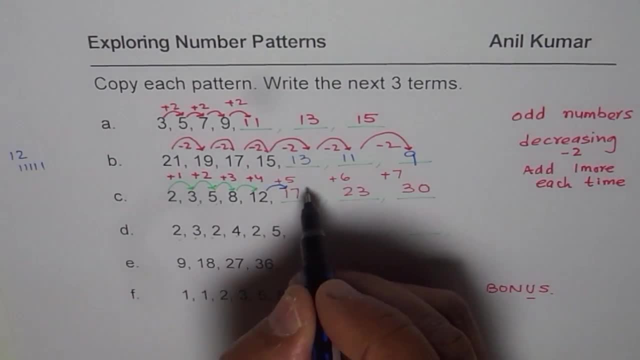 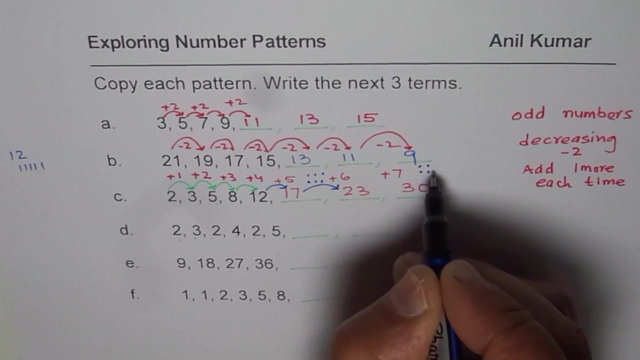 correct. And then you have to add 6.. So 17,, 18,, 19,, 20,, 21,, 22,, 23.. So adding 6,, we get 23.. Now to 27,, you say 23,, 24,, 25,, 26,, 27,, 28,, 29, and 1, 30. So these 3 dots, 7 dots you added to get 30. 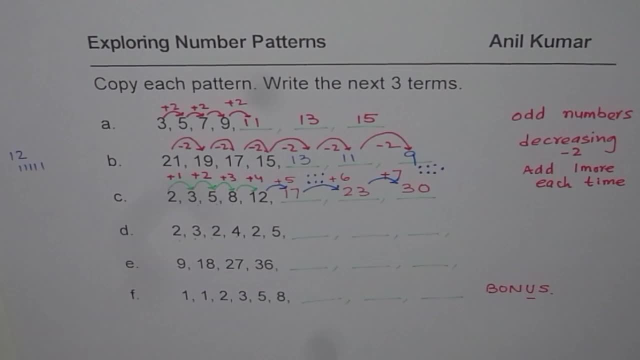 So that is how you can get the next number right Now. what we have here is 2, 3, 2, 4, 2, 5.. Hmm, how to do this one? That seems to be complicated. What you notice here is: 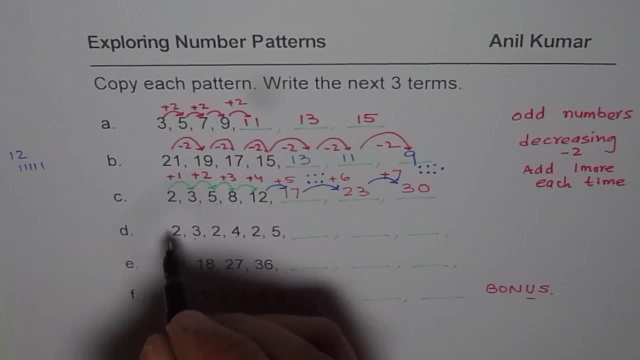 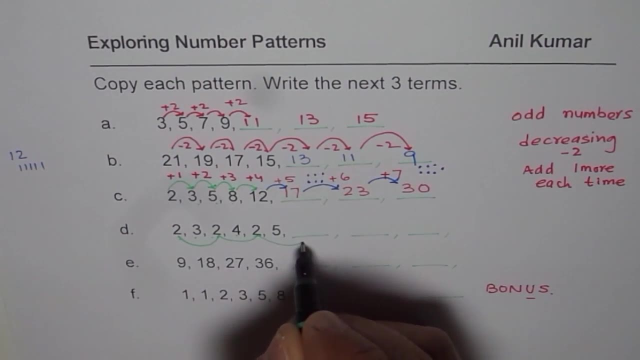 that this 2 remains constant. So alternate 1, 2. You skip and then write 2. And then you skip, and then write 2. And then you skip and write 2.. That helps correct. And how about? 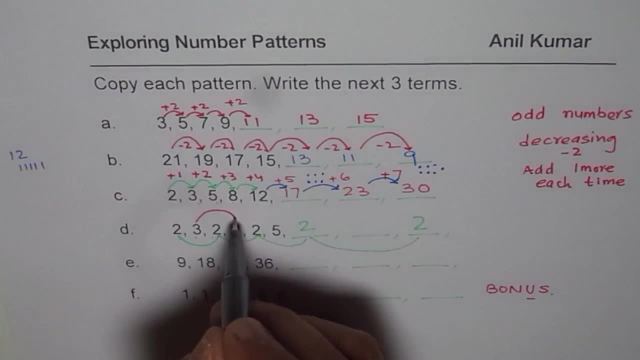 this number. Well, let's look into this: 3,, 4,, 5, and then you should get 6.. So that is how you can do this particular pattern. I hope you find it interesting. Correct, Okay, Now this one is 9,, 18,, 27,, 36.. How do we get this? It is 9 times table, right, So you are. 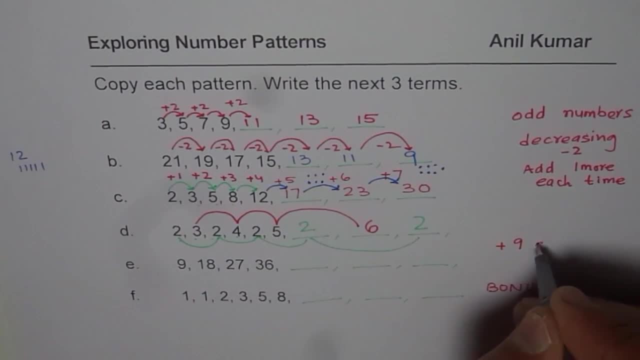 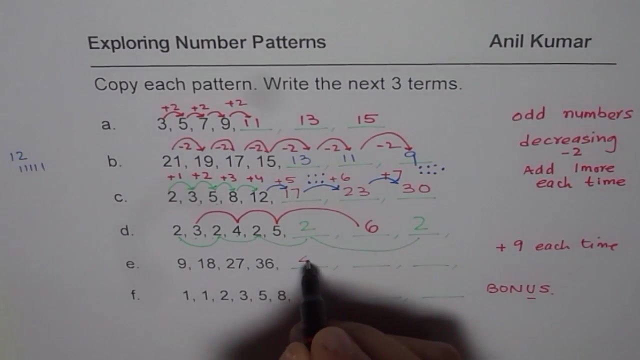 adding 9 each time. So you add 9 each time to get this one right. So you add 9 each time and then complete the next 3 terms. So 36, you get 45. What you also notice here is that 1's place decreases by 1 and the 10's place increases by 1.. So 45 and then. 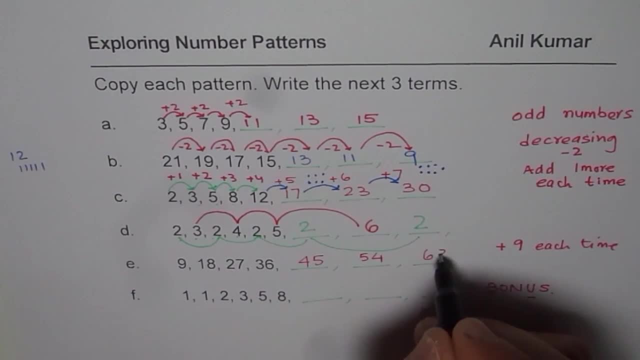 54. And then 63. So 8, start from here. 9, 8,, 7,, 6,, 5,, 4, 3 and 0, 1,, 2,, 3,, 4,, 5,, 6.. Do you?